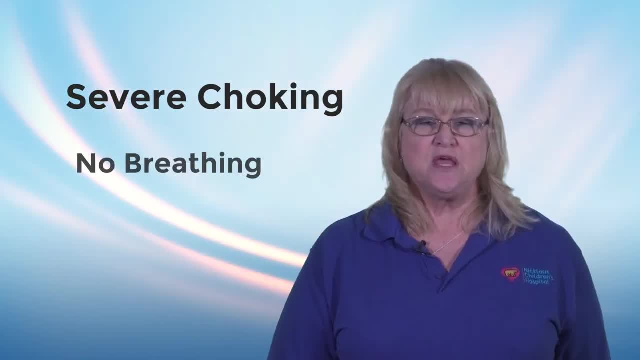 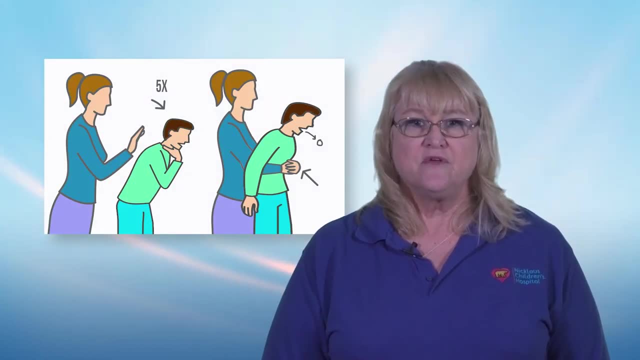 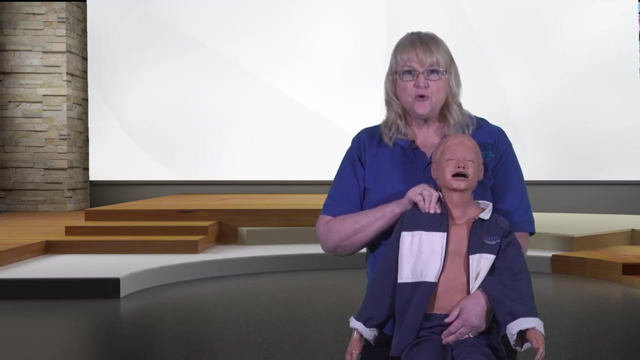 In severe choking the child is not able to breathe, to cough or to speak. Your quick response to choking can save your child's life. You will need to get the object out so the child can breathe. If you think the child is choking, ask the child. 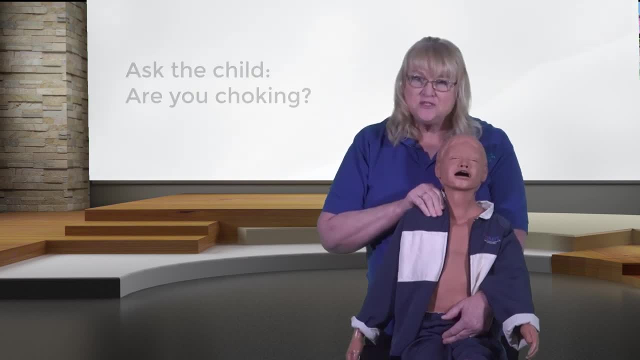 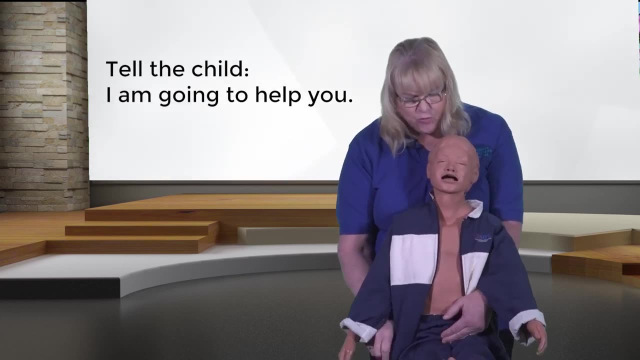 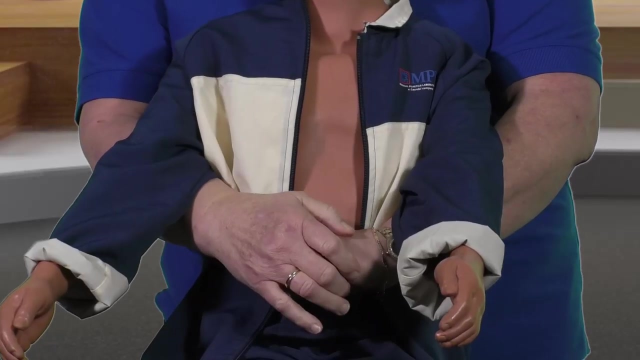 Are you choking? Are you choking? If he nods, let them know you're going to help them. I'm going to help you. Get behind the child, Reach your arms under the child's arms, Put one fist just above the child's belly button and grab that fist with your other hand. 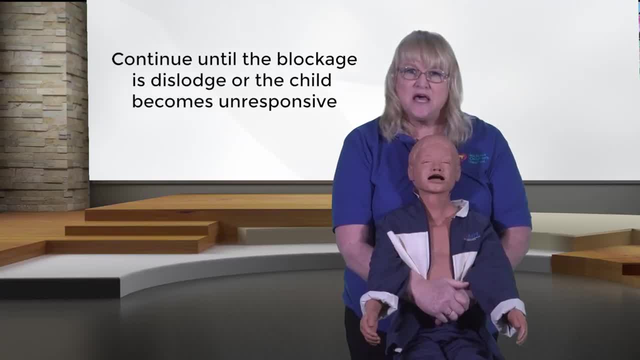 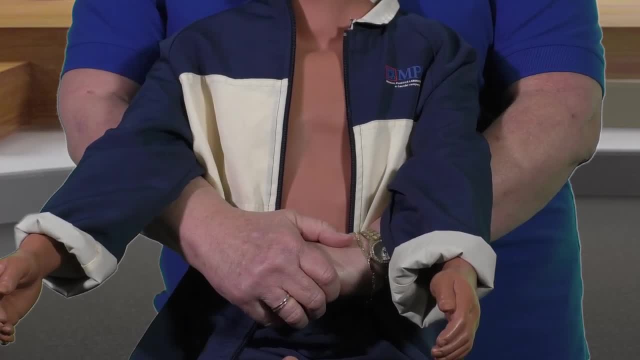 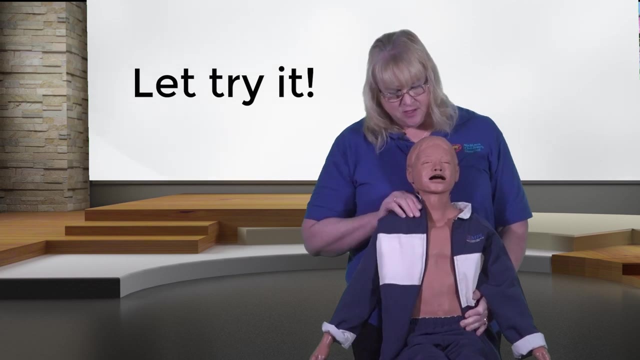 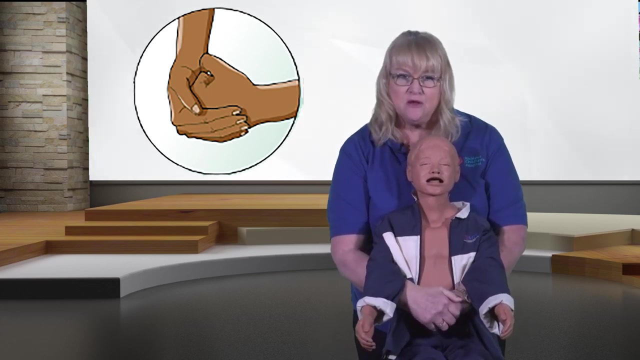 Give quick upward thrust until the object comes out and the child can breathe or cry, or until the child becomes unresponsive like this. Let's try this together. Are you choking? Are you choking? I can help you. One fist just above the belly button, grasping the other. 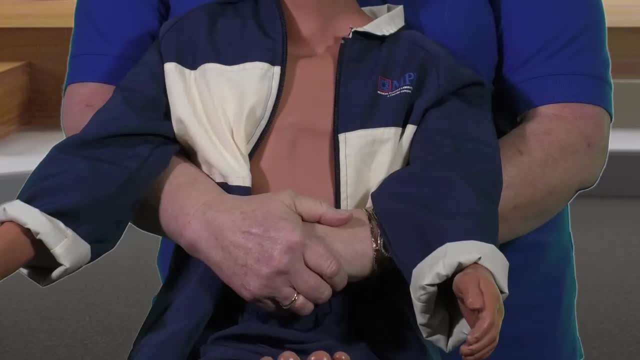 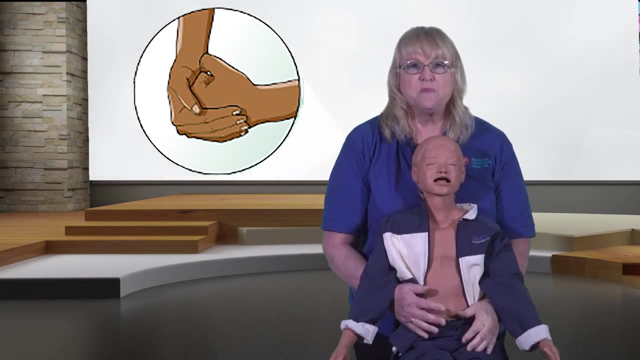 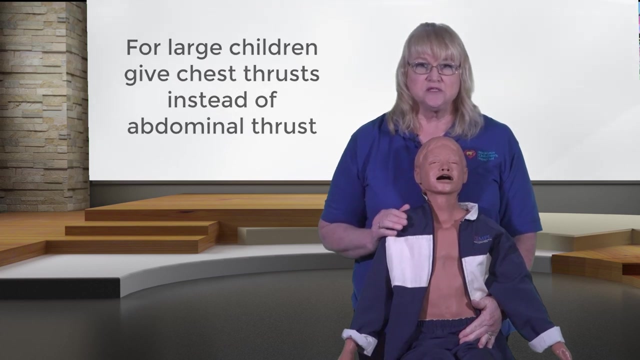 Continue with the upward thrust until the object comes out and the child can breathe or cry, or until the child becomes unresponsive. If the choking child is very large, you may give chest thrust instead of abdominal thrust. If the choking child is very large, you may give chest thrust instead of abdominal thrust. 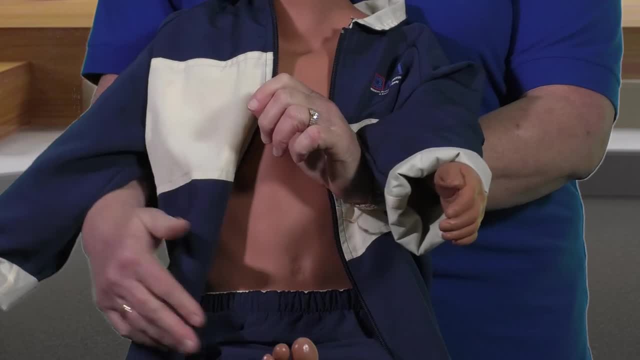 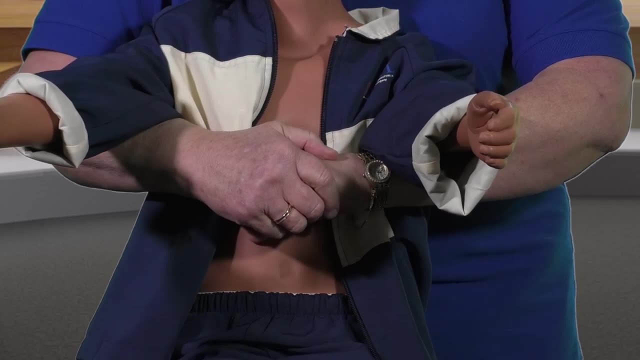 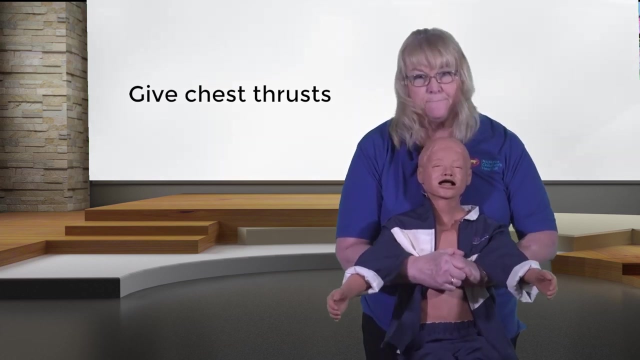 To give chest thrust. reach your arms under the child's arms, placing your hands on the lower half of the child's breastbone. Pull straight back until the object comes out or the child becomes unresponsive like this. Let's try this together. 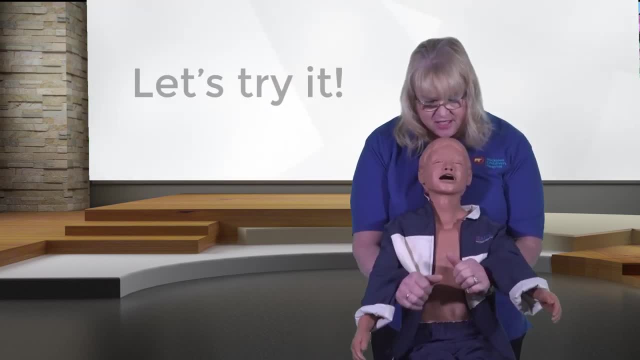 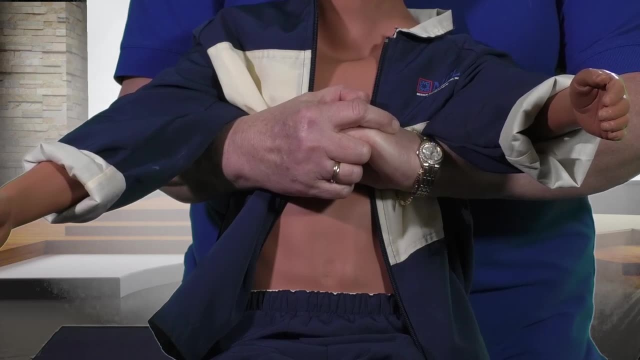 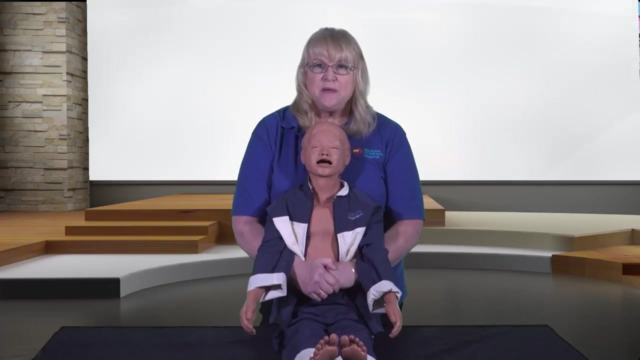 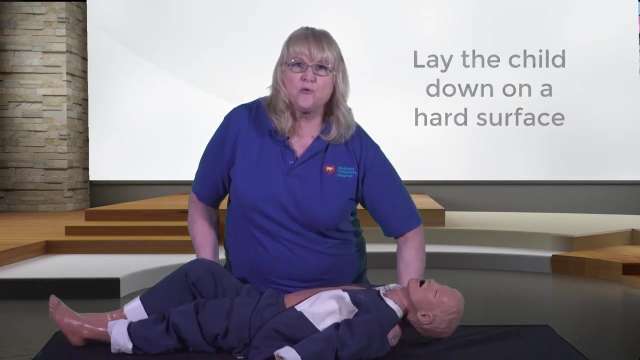 For a large choking child. hands under the child's arms, hands over the lower half of the breastbone, pulling straight back. Pull straight back until the object comes out or the child becomes unresponsive. If the child becomes unresponsive, lay the child down on a hard surface such as the table or on the ground. 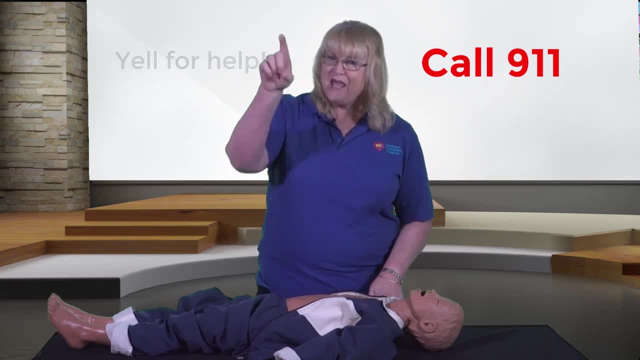 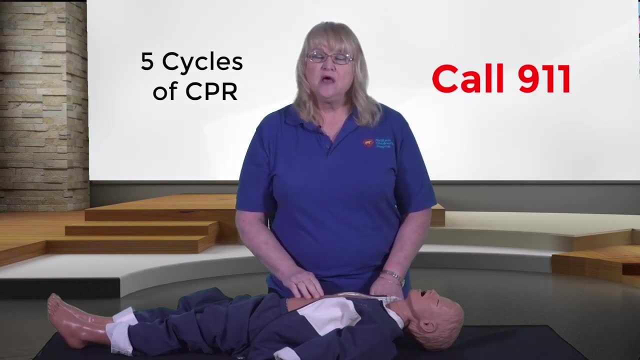 Yell for help. Help, Help Someone. call 911.. Hey you in the blue shirt. call 911.. If you're alone, you'll need to provide five cycles of CPR. then call 911.. Keep the phone on speaker so emergency staff can guide you. 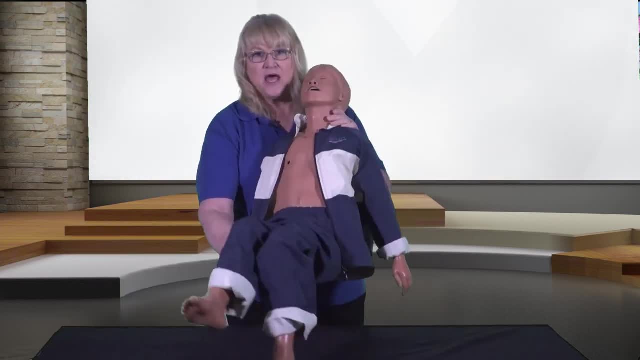 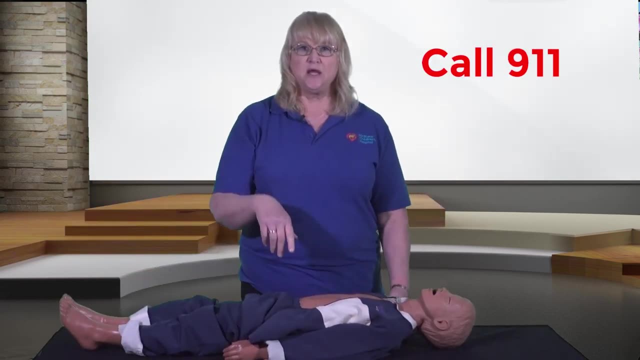 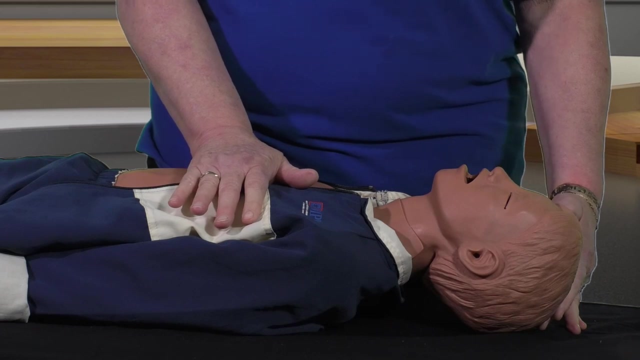 Let's try this together. Place the child. Let's place him on a hard surface. Help, Help. I need help in here. Somebody call 911.. We will start with compressions, Thirty compressions. Place the heel of one hand on the lower half of the child's breastbone. 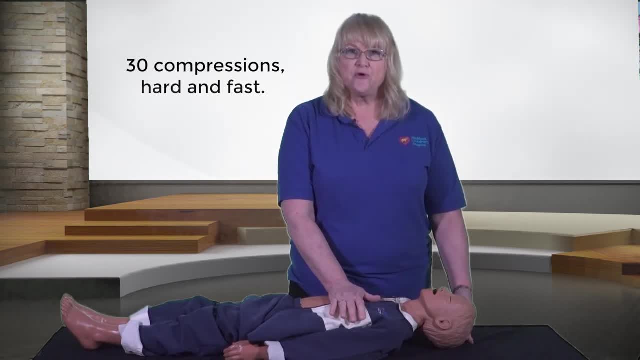 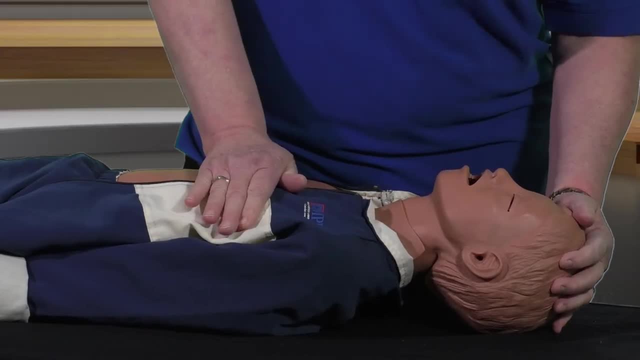 Push hard, Push fast. Counting out loud to a count of 30.. One, Two, Three, Four, Five, Six, Seven, Eight, Nine, Ten, Eleven, Twelve, Thirteen, Fourteen, Fifteen, Sixteen. Seventeen, Eighteen, Nineteen, Twenty One, Twenty Two, Twenty-three, Twenty-four, Twenty-five, Twenty-six, Twenty-seven, Twenty-eight, Twenty-nine, Thirty, Twenty-seven, Twenty-eight, Twenty-nine, Twenty-ten. 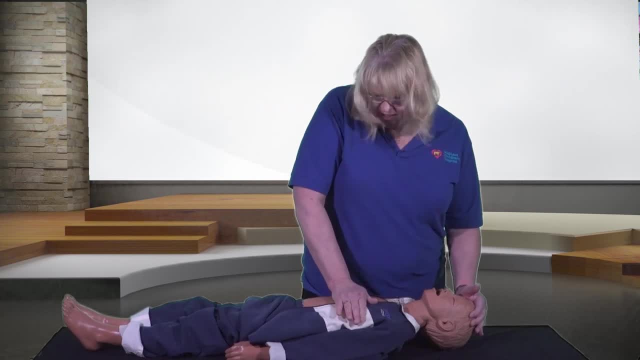 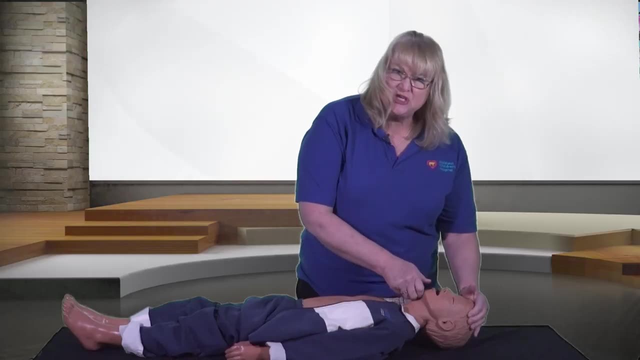 Twenty-seven, Twenty-eight, Twenty-seven, Twenty-seven, Twenty-eight, Twenty-nine, Twenty-seven, Twenty-eight, Twenty-nine, Twenty-thirty. Now you'll have to check the airway for any objects. Head tilt, chin, lift One hand on the child's forehead. 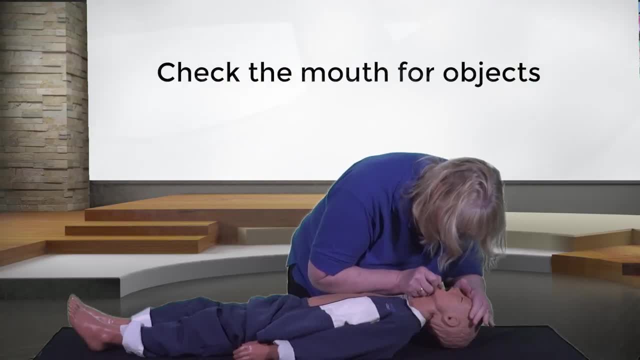 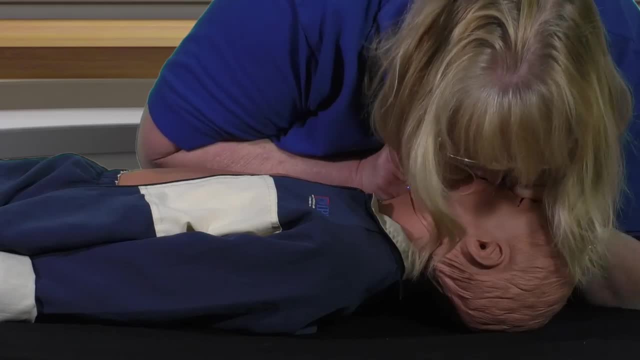 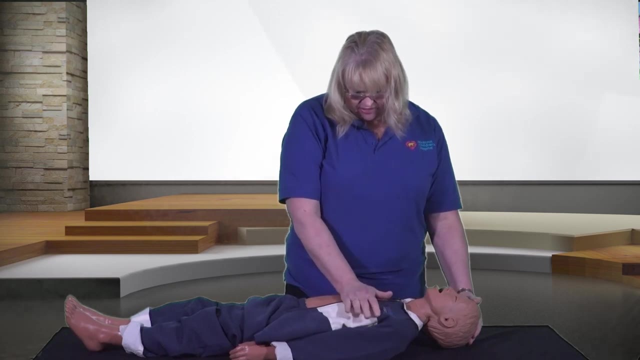 Two fingers on the chin to tilt the head back. Check the mouth to see if you see any objects. If no objects are seen, reach the child's nose, cover the child's mouth and attempt to breathe. If air does not go in, you need to repeat the chest compressions. 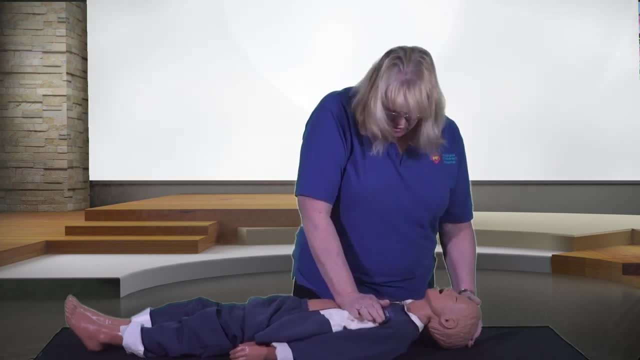 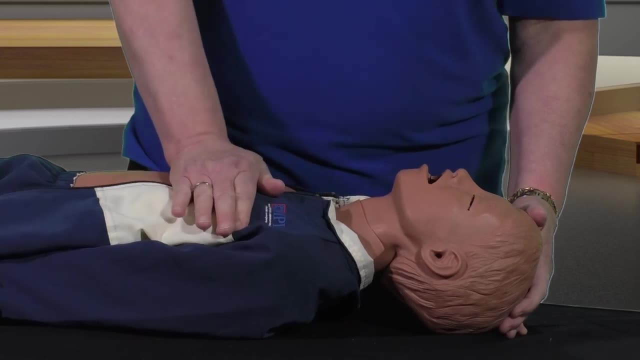 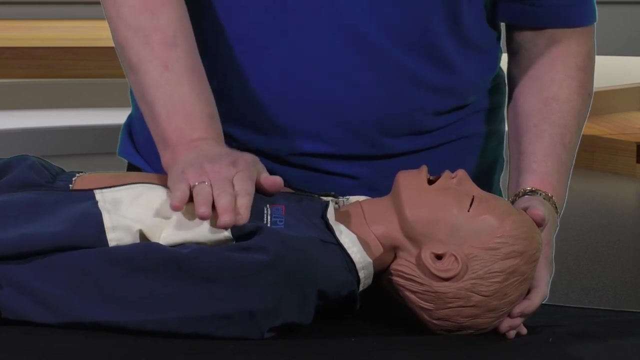 Thirty compressions Lower half of the breastbone: One, Two, Three, Four, Five, Six, Seven, Eight, Nine, Ten, Eleven, Twelve, Thirteen, Fourteen, Fifteen, Sixteen, Seventeen, Fifteen. 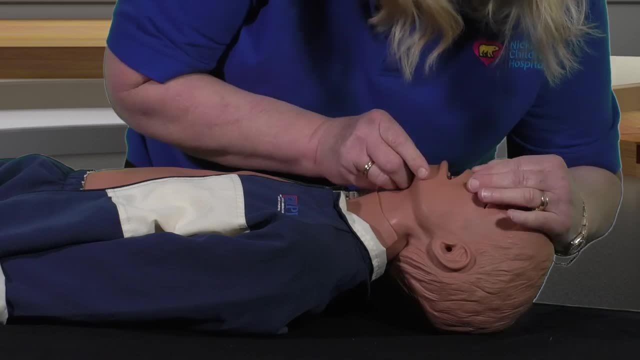 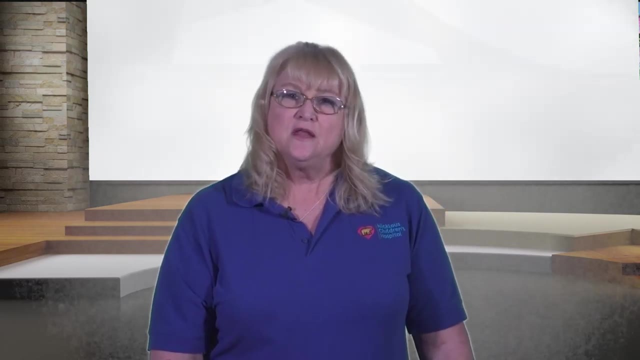 Thirteen, Fifteen, Sixteen, Eighty, Thirty, Less than a minute. We're going to do the airway Head tilt, Chin lift, Checking for objects. No objects are seen. Pinch the nose, Attempt to breathe. 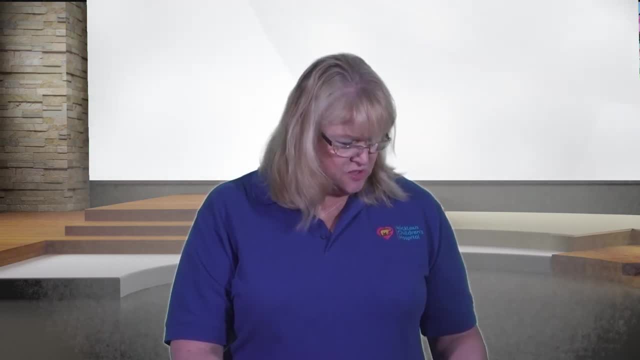 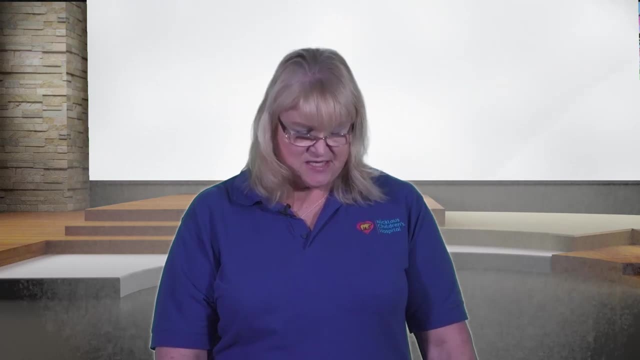 Repeat the process over and over again: Thirty compressions, Opening the airway, Checking for objects, Attempting to breathe, Over and over until the child wakes up and can cough or cry or the emergency staff arrives to help you. This completes our video on how to help a child that is choking. 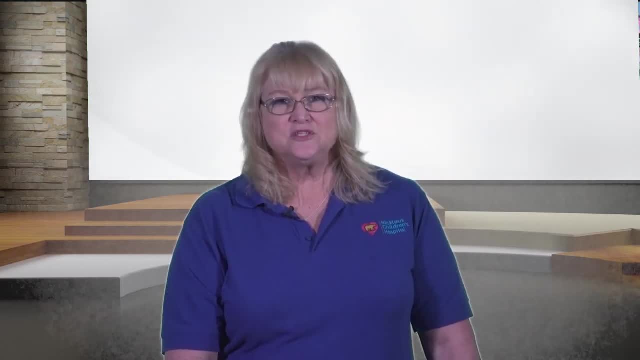 is choking. On behalf of all of us at Nicklaus Children's Health System, we hope you found this instructional video helpful. Thanks for learning with us.